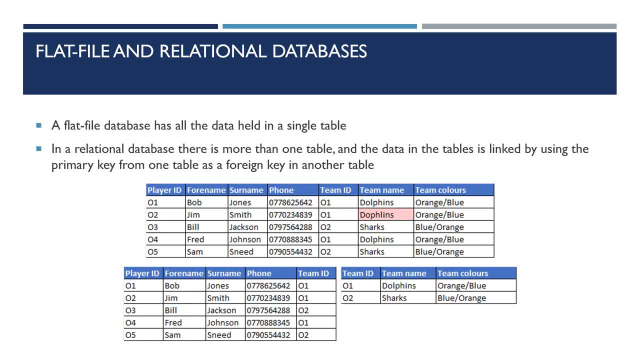 database with a table for players and a table for teams. We've included the team ID field in the player table as a foreign key in order to create a link between the two tables. This means you would still be able to find out the team name for any player. that's in. 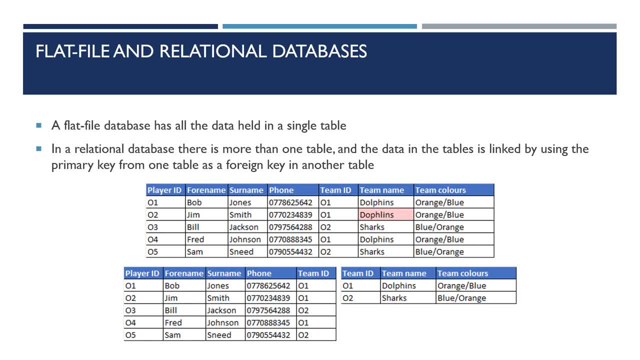 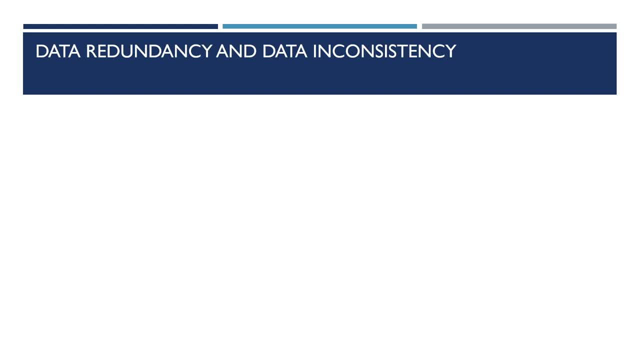 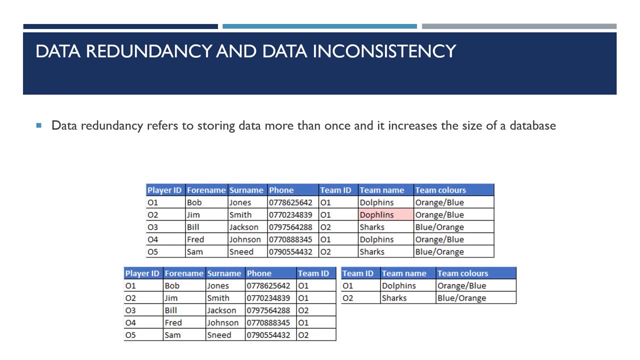 the player database and their team colours because of the link that's been created. Relational databases can help us to overcome the problems of data redundancy and data inconsistency that are found in flat file databases. Data redundancy refers to storing data more than once. This obviously increases the size of a database. For the simple example of a flat 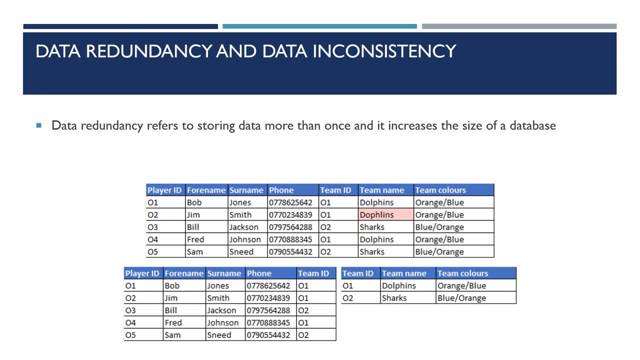 file database we're looking at. it may not seem like that much, but for a large firm with thousands and thousands of records, it can make a very big difference to the size of the database they're trying to manage. Data redundancy can lead to the other problem. 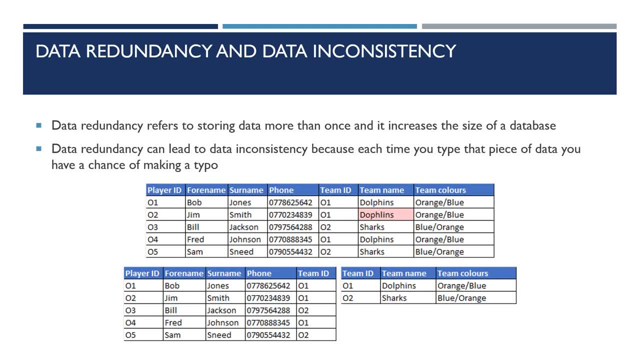 data inconsistency. This is because each time you have to type in that same piece of data, you have a chance of making a typo. This has led, in our example of our flat file database, to one of our players having dolphins misspelled as their team name. If we were trying to find 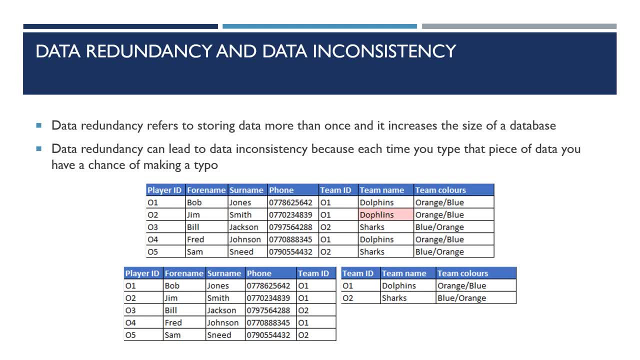 out the problem. in a flat file database we'd have to go through one line at a time to fix them up. If the team name was wrong in a relational database, we'd just fix it once in the team name field in the teams table. Inconsistent data could lead to inaccurate results from 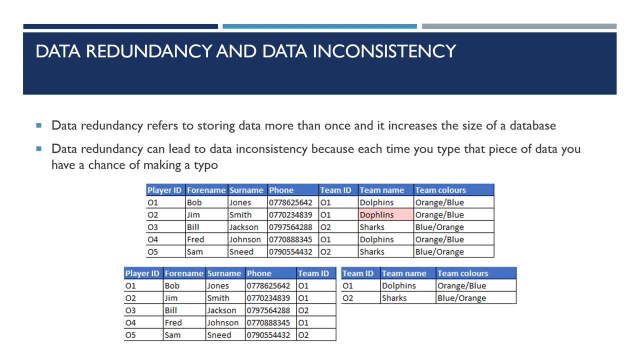 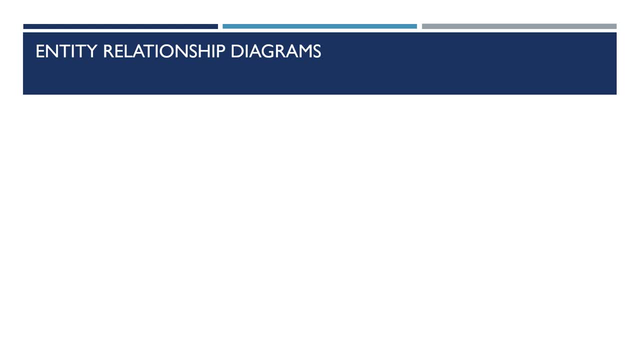 queries where, for instance, Jim Smith might not be identified as being in the Dolphins team. When designing a database, it helps to first display the relationships between each of the tables you intend to use. If you're trying to find out the problem in a flat. 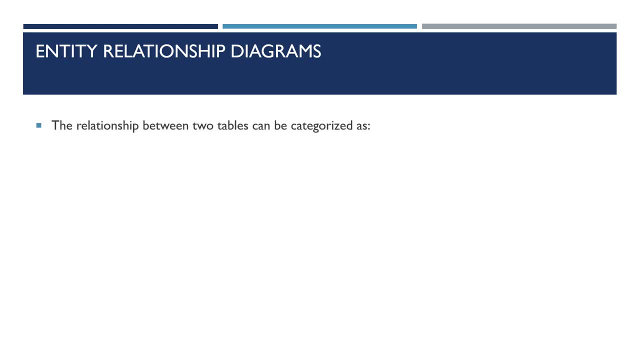 file database, you'll need to look at the relationship between the two entities. Relationships in the database can be categorised as one-to-one, one-to-many or many-to-many. To work out what kind of relationship you're looking at between two entities, you should consider 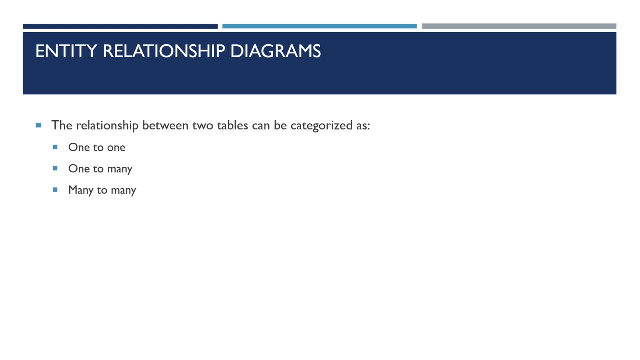 the relationship from both ends. For instance, a student and report card have a one-to-one relationship. This is because any one student will receive one report card and any one report card will be for only one student. This is because any one student will receive one report card and any one report card will.